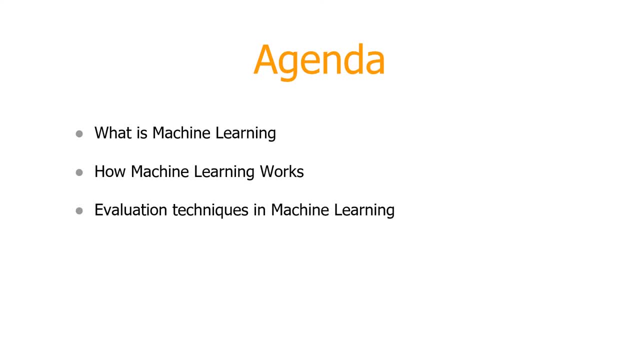 learning. So let's get started. We have lots of data generated every hour than ever before. So machine learning, in very simple terms, is nothing but extracting knowledge from those data stores using an algorithm so that we could make better predictions about our future. And broadly, there are two kinds of machine learning problems: the supervised machine. 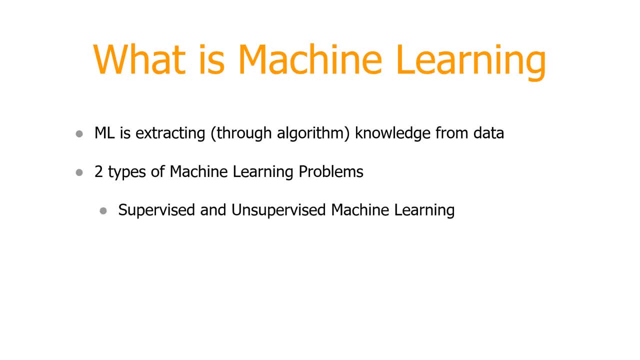 learning and the unsupervised machine learning problem. In this video, we will discuss about supervised machine learning. In supervised learning, both the input and the decision making are based on the data that is being generated. In supervised learning, both the input and the decision making are based on the data that is being generated. In supervised 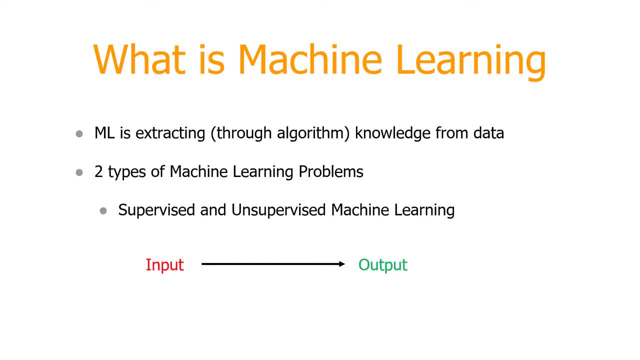 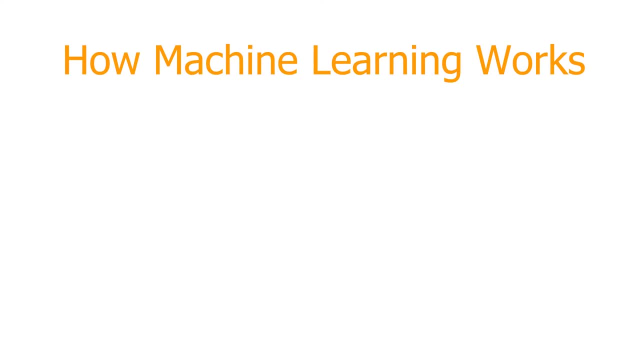 learning. both the input and the decision making are based on the data that is being generated And output are provided, and our model tries to learn the relationship between the two. Let's understand how machine learning works with a simple example. Nobody can define: oh, oh, no, oh oh. 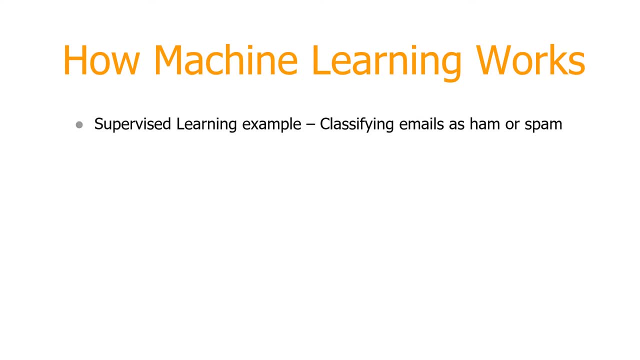 eh mm. One of the classic supervised machine learning problem is email classification in production, ie to classify whether an incoming mail is a ham or a spam. Suppose we have a dataset that contains historical data about emails. Each record in the dataset is an observation. 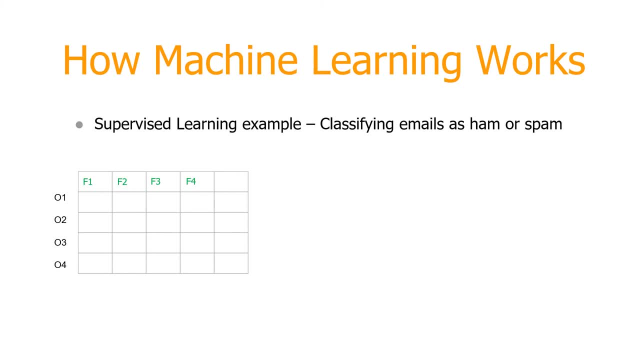 And each column in the dataset is a feature. The features for email classification could be the length of the email or the presence of a certain hyperlink or the presence of some words that are very common in spam emails. This is the input to the machine learning algorithm and is called the feature matrix. 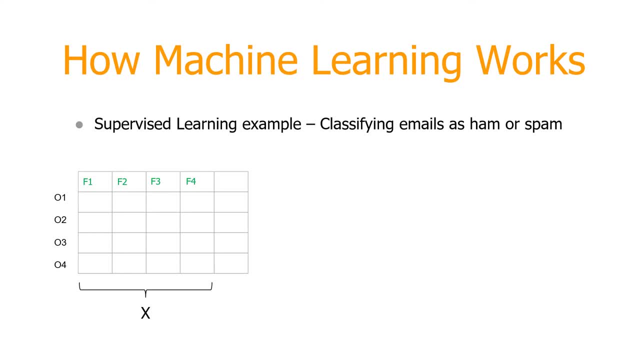 X. In supervised machine learning, you also have the labels, which is the output of the machine learning algorithm, as it predicts whether an email is a ham or a spam, based on the input features. This output is called the response vector Y. So once you have this label dataset, you can choose any algorithm, for example a KNN or. 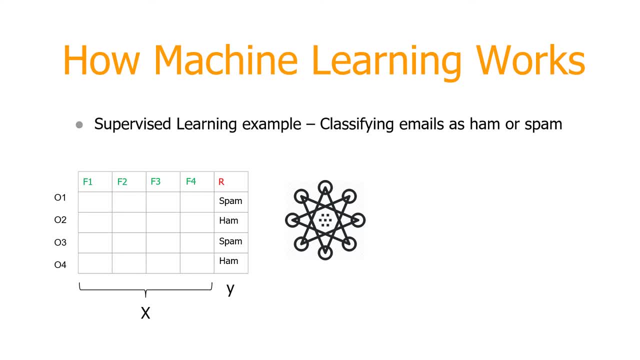 a logistic regression or a random classifier to train the algorithm. with this training data, The model looks at the input data and learns the parameters or weights of the input features that would accurately predict the output response, Or, in other words, it tries to find the relationship between the input features and the output. 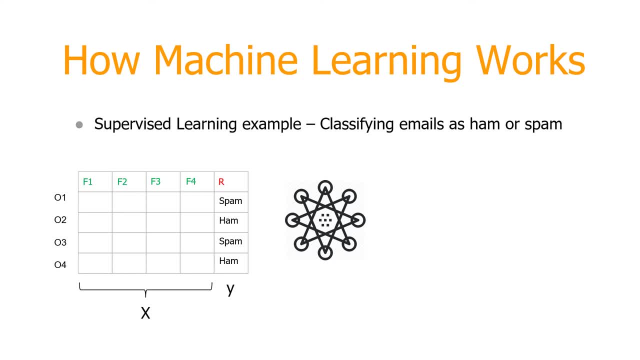 response. Then it tries to construct a model, or you can think of like an equation, where it can predict the output response as a collection of input features. So this is the output response. So when I say the model learns the parameters, it learns the different weights of the features. 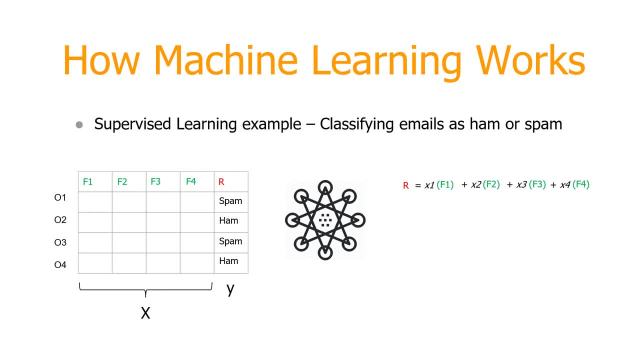 that need to be used to predict the response And, based upon the value of R or the response, the model will conclude if a particular email is a ham or a spam. Note that some features have a very positive correlation to the response. For example, I am almost certain that if there is an image, 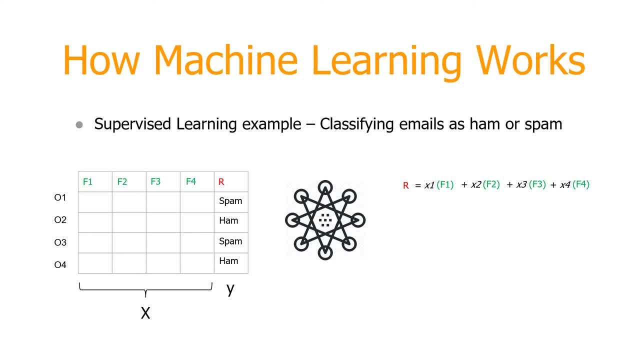 Embedded in an email, it is most probably a spam. So this feature gets a weight close to 1.. And some features have negative or even no correlation to the response and their weights will be determined accordingly from the training data set. As I said, you can run different algorithms on your training data to produce different. 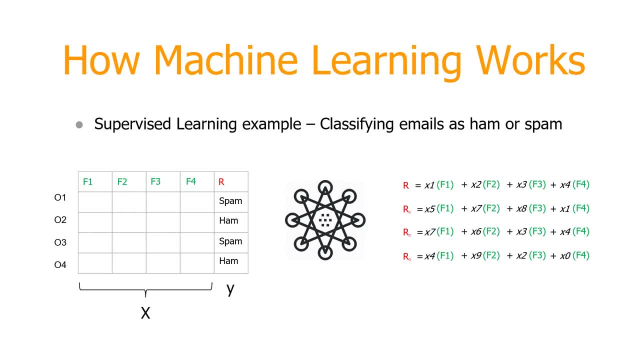 models, or one algorithm itself may produce different models, each with different parameters. So this is the first example. So our goal is to choose a model that predicts the response for the unknown data with the highest accuracy rate. So how do we know which model predicts the best if we do not know the true response values? 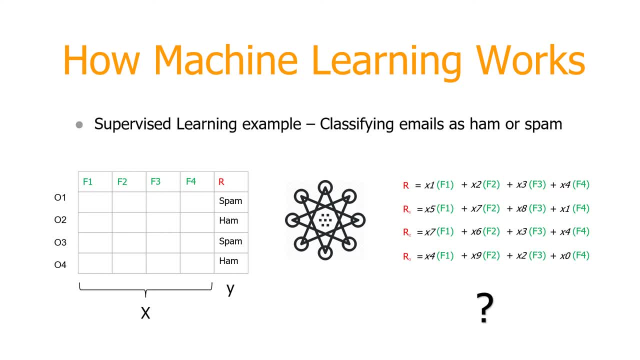 for the future data set. To select the right model for the problem, you need to evaluate the model first, So you need to understand different evaluation techniques in machine learning. But before looking at the evaluation techniques, let me tell you a few things. 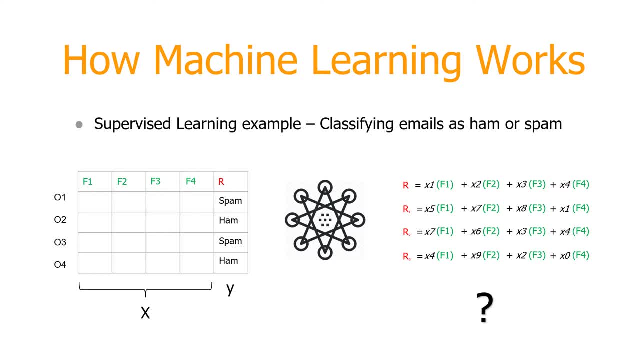 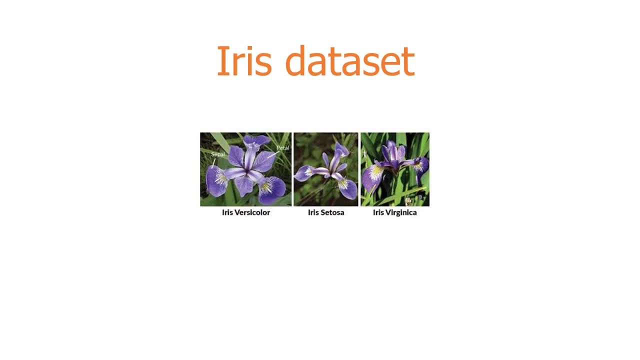 Let's first look at the iris data set that we will be working with in this video. It is a very popular data set, provided with Skykit learn that predicts the species based on the length and width of sepals and petals. So let me go to Jupiter and import the data set. 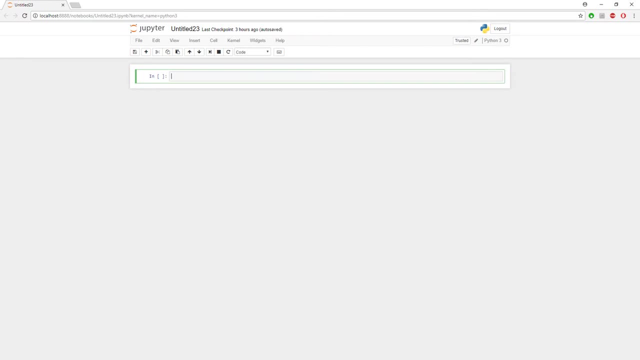 So let's go to Jupiter and import the data set. The iris data set is a very popular data set. The iris data set is provided in sklearn, So let me import load underscore iris function from data sets module and save the iris data set in the variable iris. 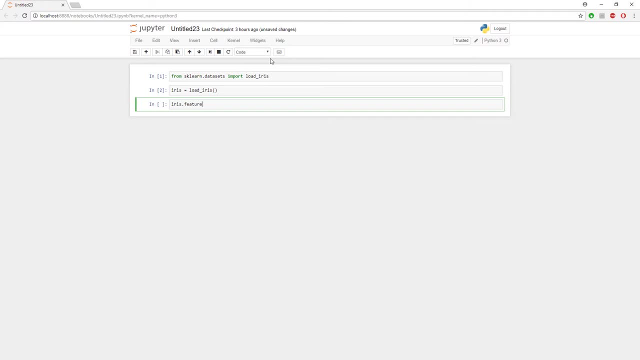 If you write iris dot feature underscore names you will get the feature matrix. To see the response values, just enter iris dot target names. So this is a classification problem, because you are predicting if each observation is a setosa or a versicolor or a virginia using the dimensions of the species. 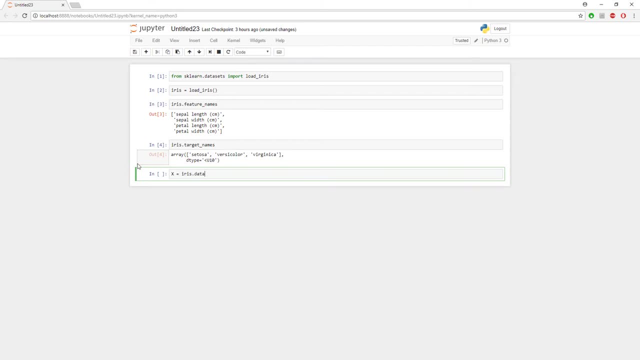 So let's extract the feature matrix and store in variable x and store the response vector in variable y. Let's check the shape of the x matrix. There are 150 different observations in this data set and it has four different features, And y contains 150 response values. 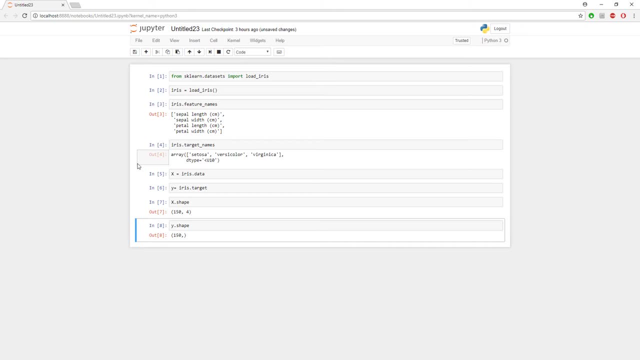 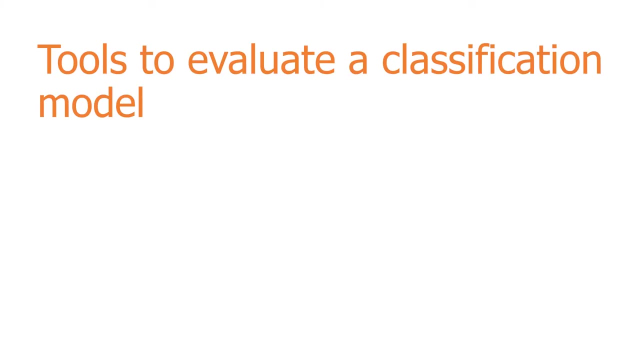 Now that we understood what is within our data set, let us go to slides to look at the different options to evaluate a classification model. There are several tools to evaluate a classification model. They are training and testing the model on the data set. There are several tools to evaluate a classification model. 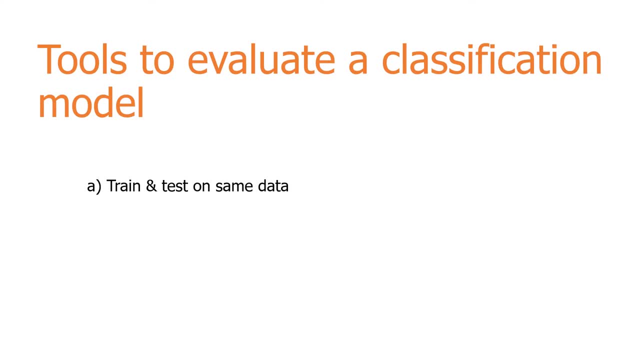 They are training and testing the model. on the data set. You can array diodes to make your testing model run. You can also use a specific test plate and trunking tool, but during the test We can define a capitalization and costing, data chunking and constant so that it would be even more. 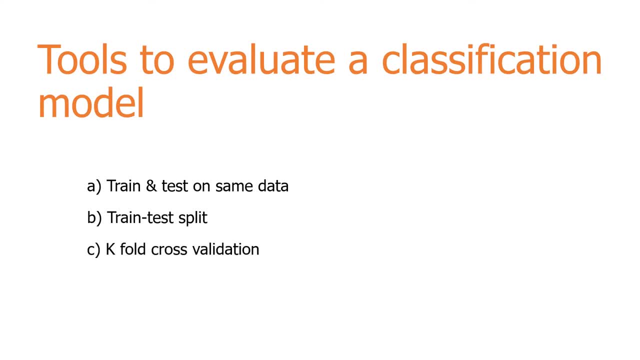 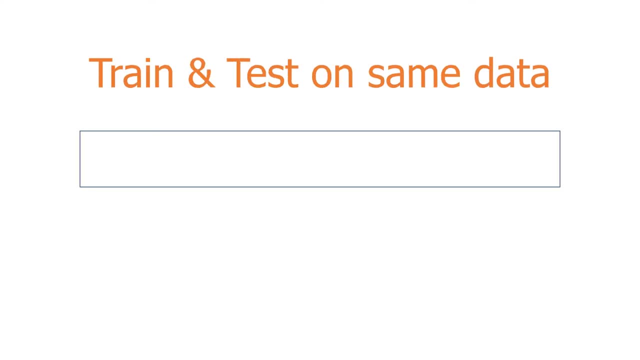 efficient and standard. Let us look at training and testing the model on the same data. We train the model directly to inform the entire dataset. Then we test it directly onto the dataset. They areHz, x and Okay, ket controls And t host. x equals to t x. 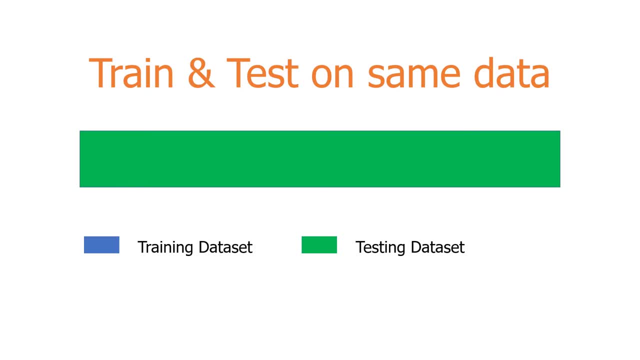 is a very basic method to check if the predictions by our algorithm is correct By testing our model on the dataset, for which you do know the true response values. you can check how well the model is doing by comparing the predicted response values with the true response values. 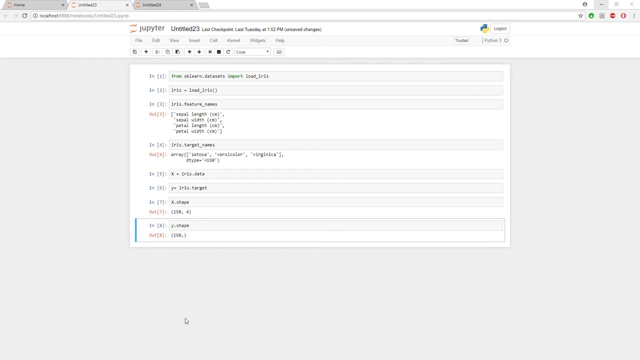 So one of the ways to evaluate a machine learning model is to train the model and test the model on the entire dataset and evaluate how well we did by comparing the predicted response values with the true response values. First let me import a random forest classifier from sklearnensemble: Random forest classifier. 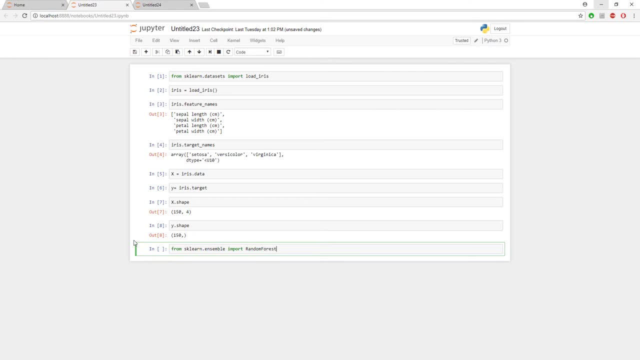 is a machine learning algorithm known to be one of the best performing machine learning models. So what I will do is, first I will use that algorithm to classify my species And before that, any process of training the model and predicting the outcome is a four step process. So the four steps are: the first step is the importing the class which we have. 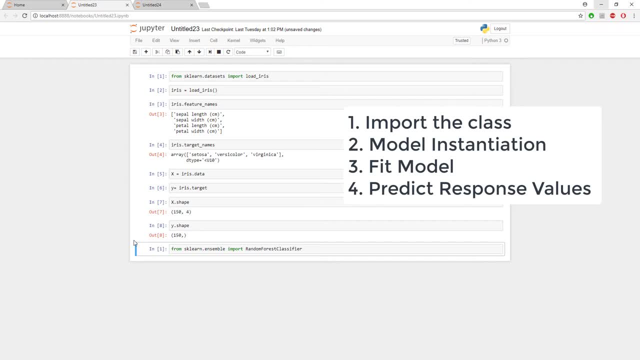 already done So we have imported random forest classifier from sklearnensemble. The second step is to instantiate the model with a default set of parameters, which we will do now, And the third step is to fit the model with the data that we have. 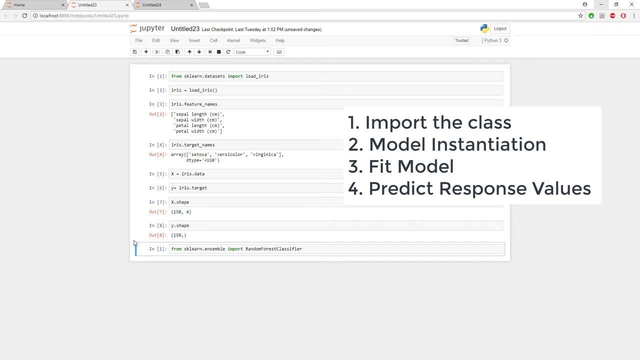 And the fourth step is to predict the model for the response values. So now let me instantiate the model. So here I will use a variable called clf. You can use any variable that really does not matter, And I am gonna say random forest classifier. 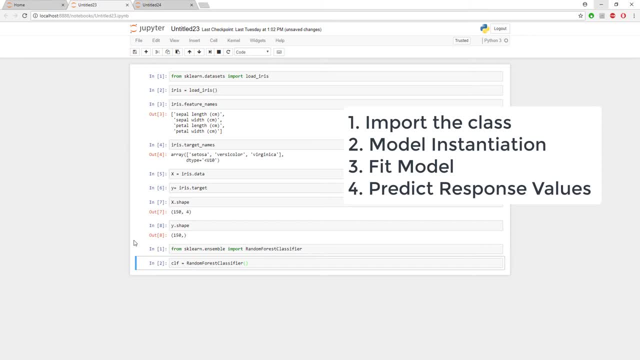 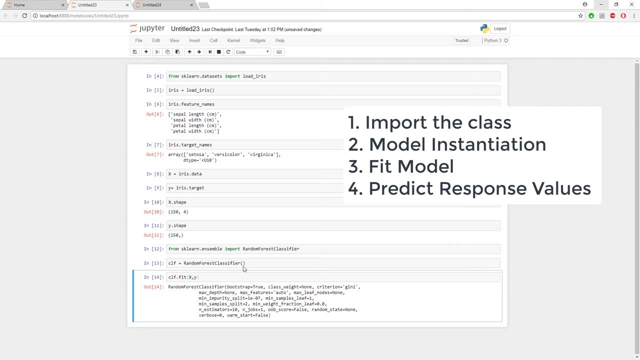 okay, so these are the different parameters and you, if you want, you can go and tinker with any of these parameters, but for this video we will not do that. we will just use the basic set of parameters that random forest classifier gives us and once you fit the model, you need to go and 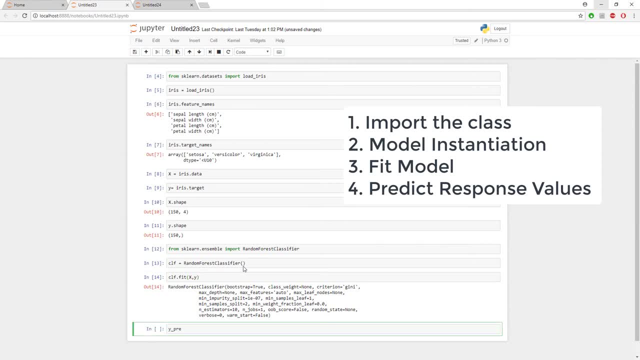 predict the response values. so what i will do is i will use the same variable, clf, and say: predict x. so it will give a list of y values for each of the x values. okay, so, for example, if there are 10 observations, the x matrix will have 10 rows and y pred will have 10 different values, but each will 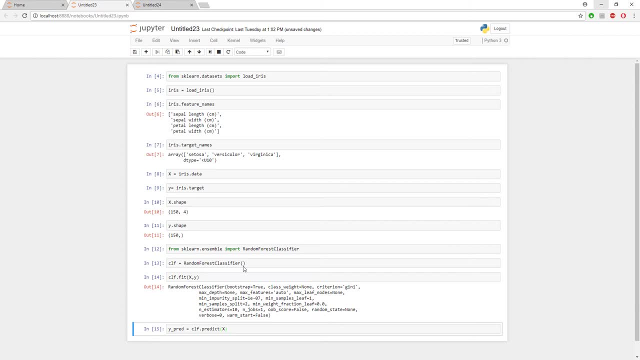 be of one dimension. now that we have the y predicted values, what we need to do is how our machine learning algorithm has predicted like: has it predicted the values the way they are? has it really predicted a setosa species as a setosa? something like that? so what you need to do is: 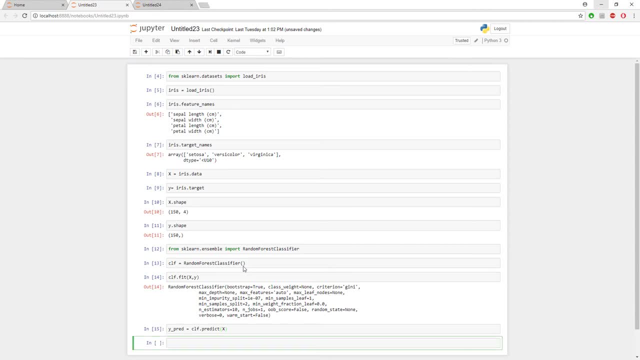 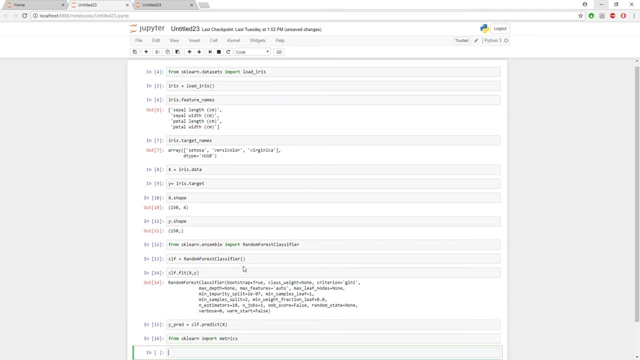 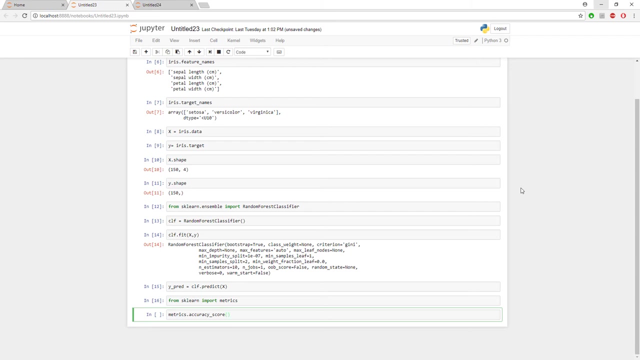 you need to calculate some kind of of a metric, some kind of an accuracy score. so for that first I will go and import metrics from sklearn and then within metrics I have this particular function called accuracy underscore score, where you will pass both the y and the y pred and note that y is the actual values and y 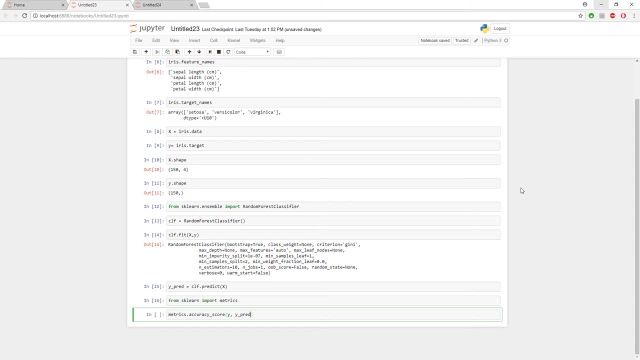 pred are your estimated values. so if you give both y and y pred, it will compare the values within y and y pred and basically it will tell what percentage of y values are matching with y pred values. and note that we are getting an accuracy score of one, which means that all our 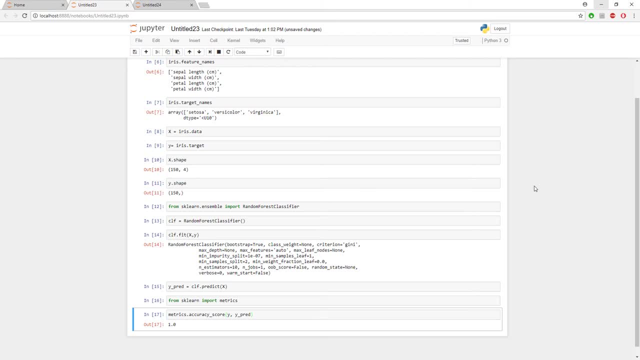 predictions are absolutely correct. our machine learning algorithm has done a terrific job of learning the relationship between the data. you now, instead of random forest classifier, what I can do is I can go and do the same thing with another classification algorithm called a logistic regression. okay, so anyway, we will not. 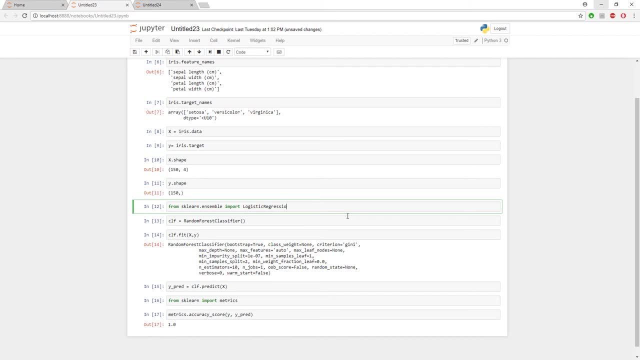 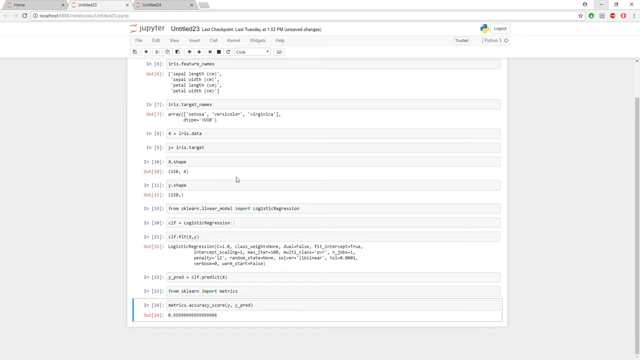 go into details about how the logistic regression works, but we will just import it and and just see how logistic regression performs and and pretty much execute all of the different statements and note that I get an accuracy score of 96 percentage, which is not really bad. but I get an accuracy score of 96, which is not really bad. but I get an accuracy score of 96. 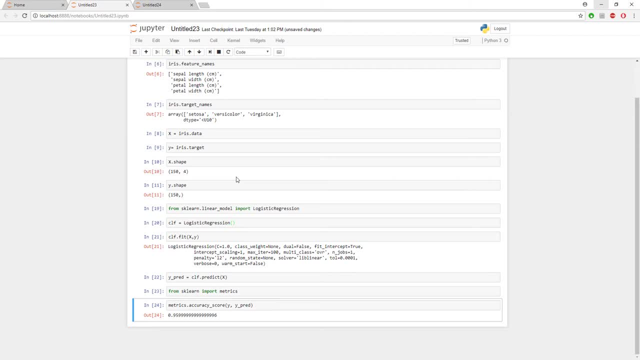 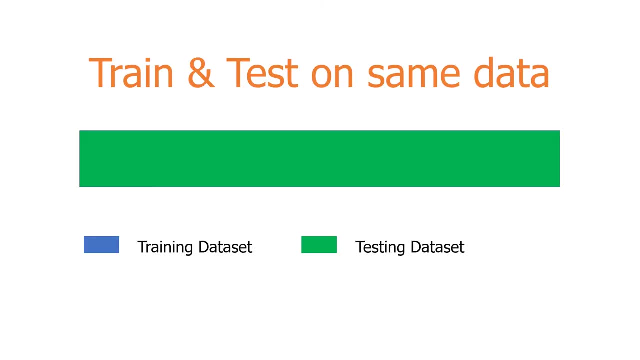 and start computing that, which is pretty bad, but probably not not as good as your random forest classifier numbers. as you can see, that is false. what you want to do what you want. so when you look at the models you are going to get, you get like a superская model, so we are going to get a much لي. 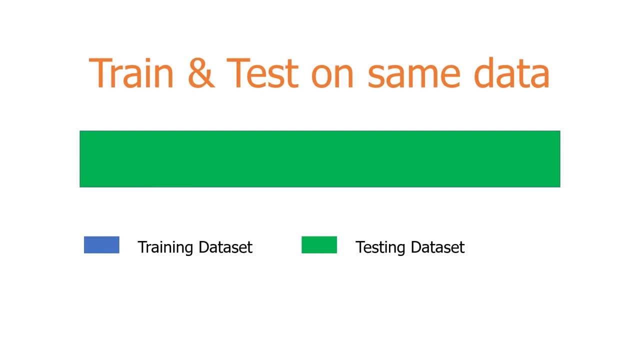 what you want to do, what you want to do, what you want to do, what we want to do. if you are going to use a thermal model, everyone needs certain kind of training. adalah model thecause. algorithm is a little bit walls of different types of models to calculate. 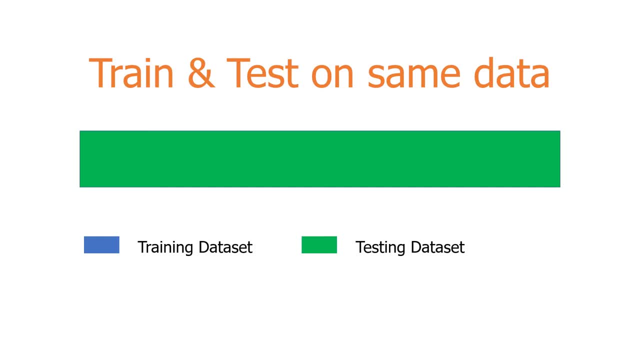 may be like the configuration model that isulu. it rewards overly complex models that won't necessarily generalize to new data that may see in the future And having a overly complex model will unnecessarily overfit the data and such a method or such a evaluation method can never be used in a production setting. 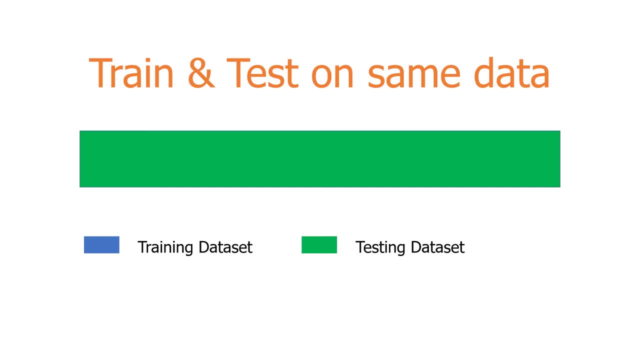 So we will move on to the next evaluation procedure, which is the train test split. The train test split is an improvement upon the previous method, where you split the data into two pieces. The first one is the training set and the second one is the testing set. 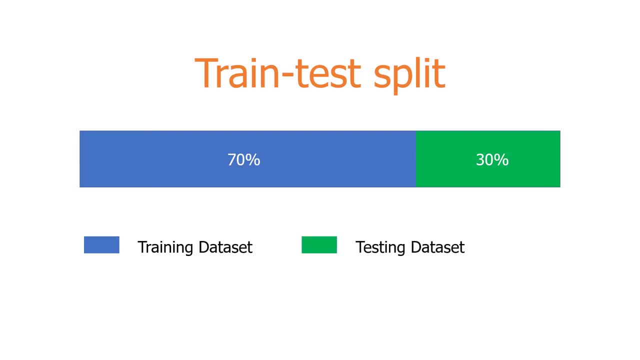 Here we train the model on the training set and test the model on the testing set and evaluate how well we did. you can split your data however you want. This is just a rough figure. you can split it either by success to 40 or 70 to 30, any way you want, and that really does not matter. so i will go to my jupyter notebook. 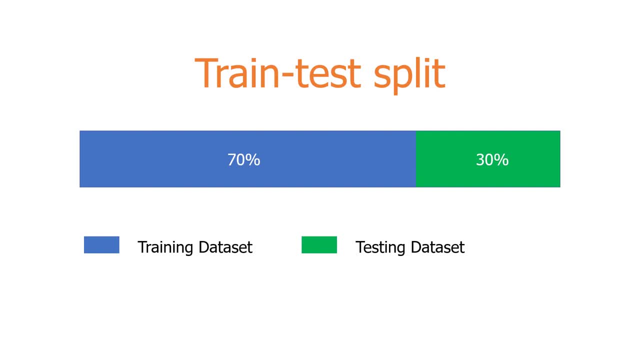 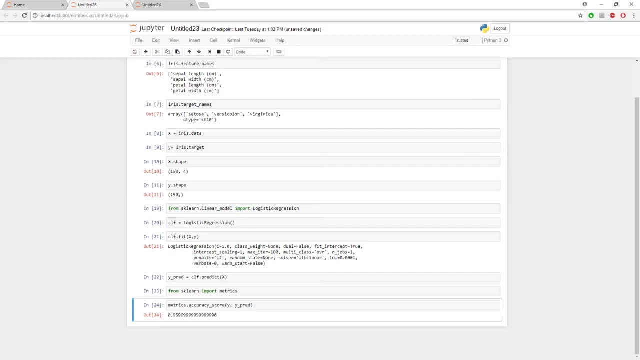 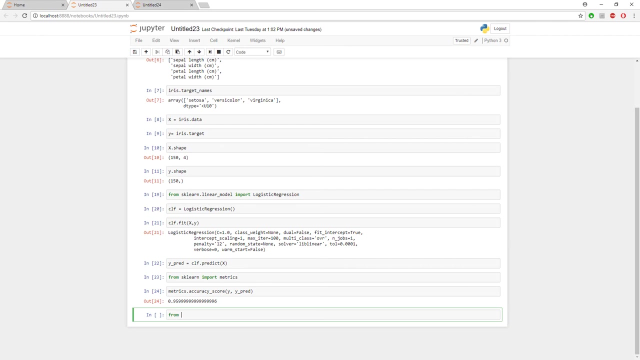 and see an example of how to split the data into training and test sets and how to do the evaluation. first let me import the train test split module. so the train test split module is available within model selection. so i will use sklearn dot model underscore selection. import. 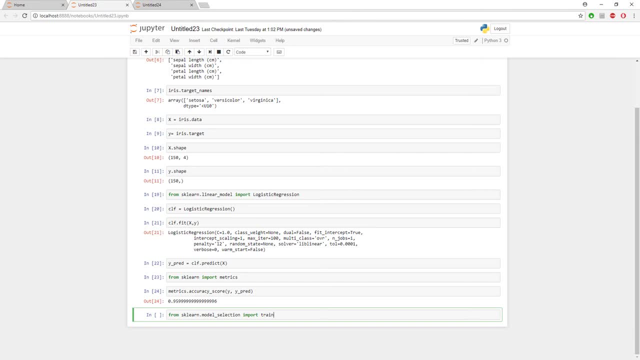 train test split. train underscore test, underscore split. and let me execute that. to split the data you need to use the function train test split. so i will say train underscore test underscore split and within the function we need to pass in the x and the y, and x is a feature matrix and the y is a response variable. okay, 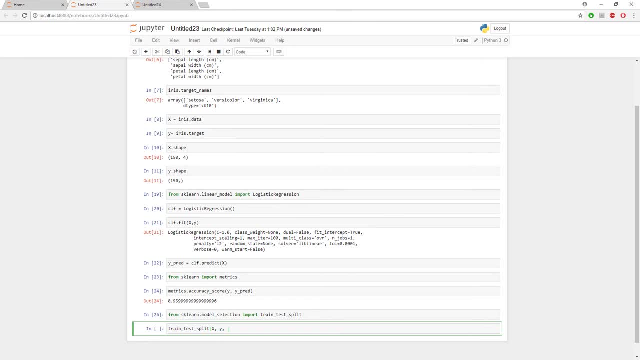 and then you need to say what is the test size. here you can say your test size as your 40, or your 30 or 20 percent, okay. so just say the test size is nothing but 0.4. okay, and we need to get the values which are coming out of this function and assign it to. 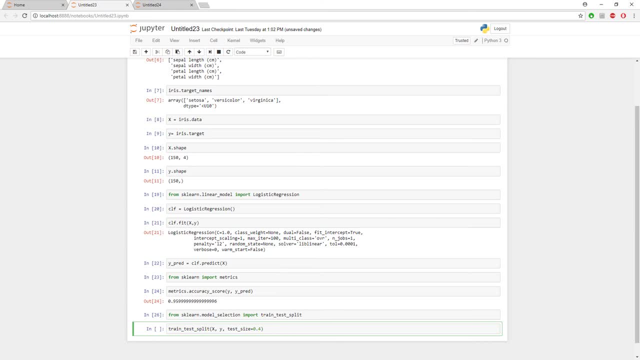 different training and testing variables. okay, so the way we do that is we just say x underscore train. okay, x underscore test, y underscore train and y underscore test. so what will happen is that, since we have 150 different observations and 150 different values for x and 150 different values for y, it will split the entirety of the data. 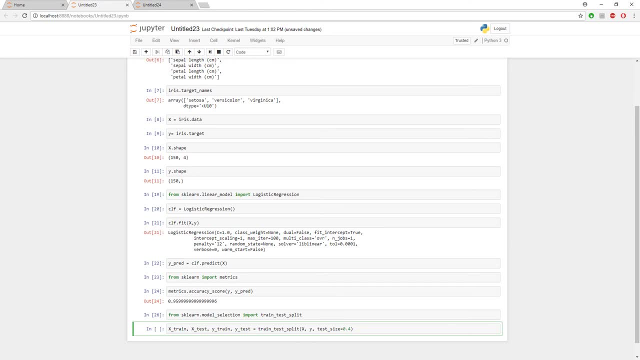 into training and testing data. okay, so the x train will have 90 observations and the x test will have the remaining 60 observations. and the same way, the y train will have 90 observations and the y test will have remaining 60 observations. so let me execute this and to show you how we have, 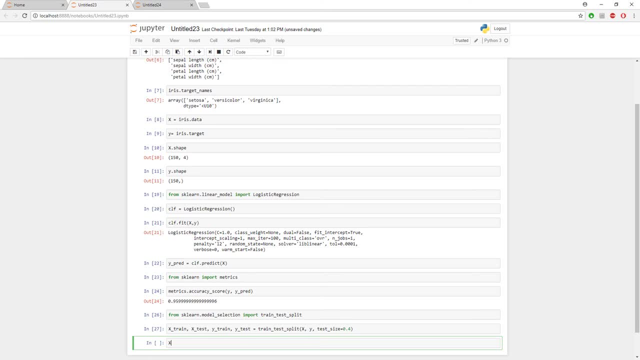 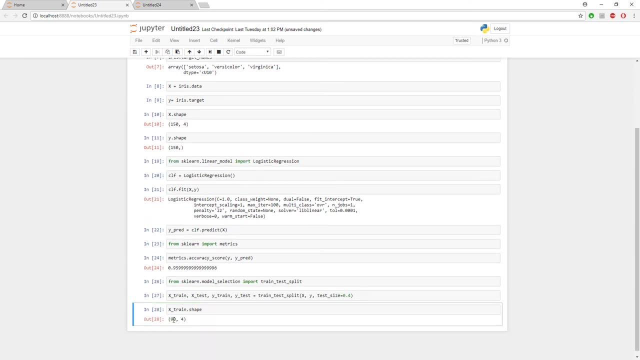 got the data. what i will do is i will execute the shape property. so i will say x underscore train dot shape and you see that we have 90 different values. okay, and these are the four different features. and if you say x underscore test dot shape, you will get the remaining 60. okay, and if i 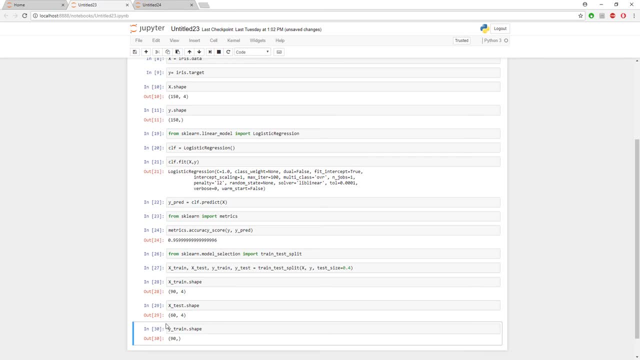 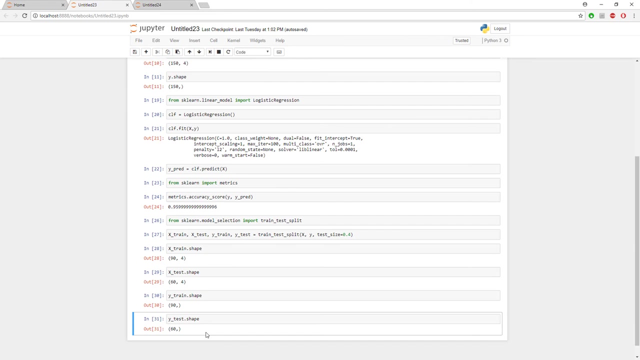 say y underscore train dot shape, i will get the first 90 values, and if i say y underscore test dot shape, i will get the remaining shape 60 values. so now, having the data split into a training and a testing set, we just need to use the training set and train our data. note that we already have initialized our variable clf to a. 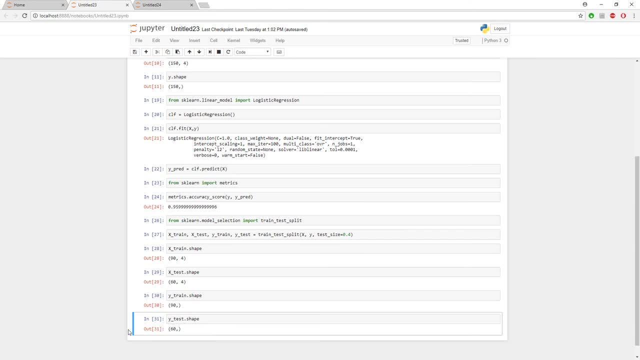 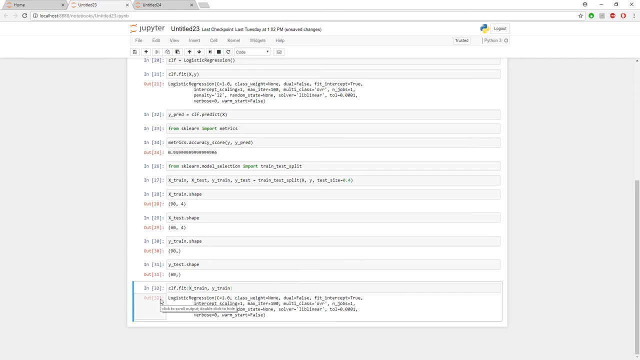 logistic regression. so i will use the same variable over here and train the new set of data. so i will say clf dot fit and i will try to fit only the training data. okay, so i will say x underscore train and y underscore train. okay, so now the clf variable has learned, the has been. 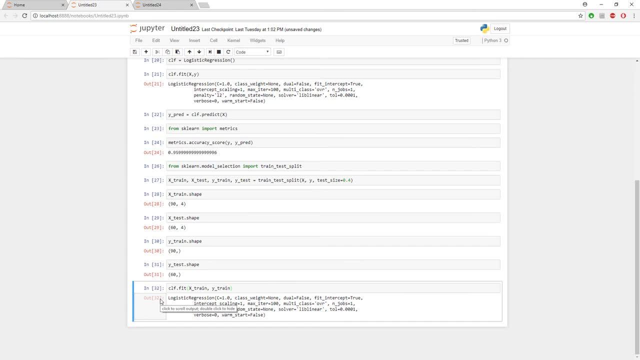 trained on the training data set. okay, so it has learned the relationships of the data within the training data set. so now we will use that clf variable to predict the values for the testing set. so i will say clf dot predict. note that this is the fourth step. 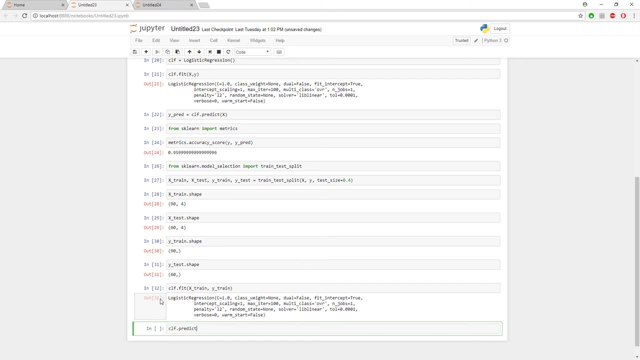 fitting is the third step and the predicting is the fourth step and i will say clf dot predict x underscore test. so basically we need to predict the y values for the testing set of x. okay, and i will store this into a variable called y underscore pred. this is called y pred because it is the 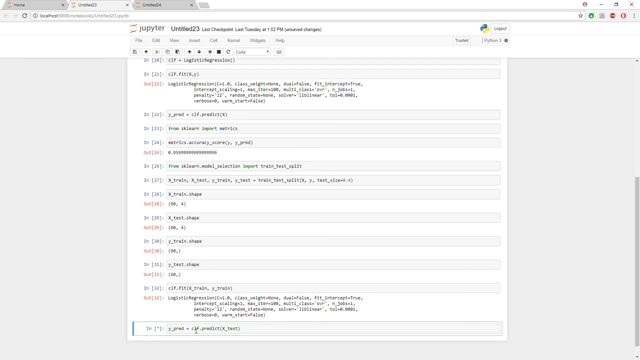 prediction of the algorithm and it is not the actual values of the algorithm or rather the actual values in the data set. so now i have y underscore pred. so i will use this same matrix module and the accuracy score. so i will say matrix dot, accuracy score and i will pass in both y test. 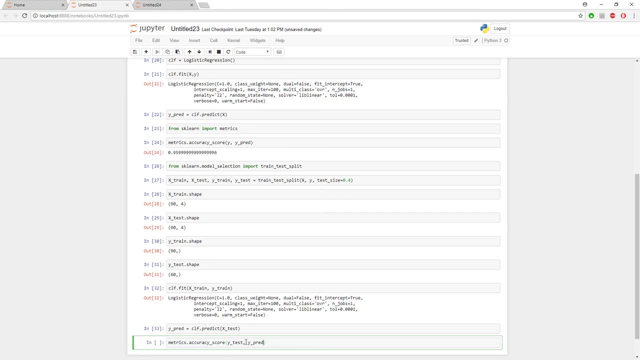 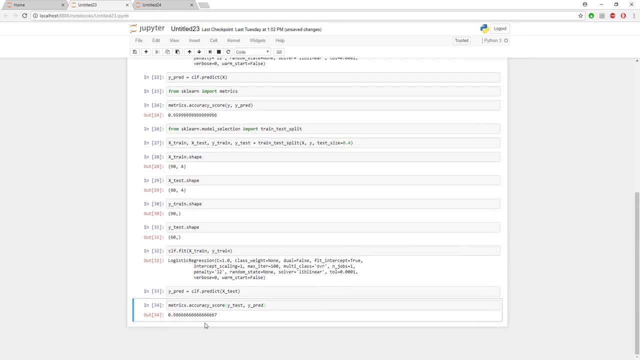 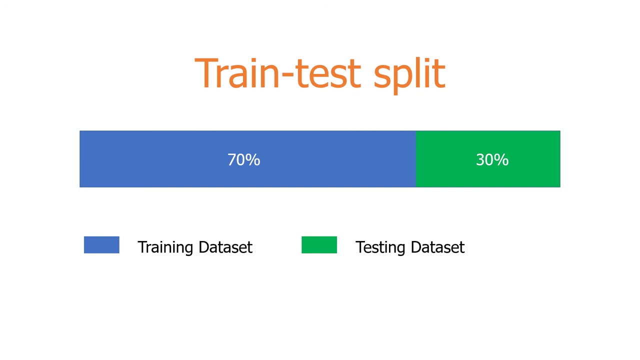 and y pred. okay, and note that y test is coming from the initial data set and y pred is the values that are being predicted by our algorithm. okay, so let me execute that and we are getting an accuracy of 97 percentage. using train test split produces what is known as a testing accuracy. testing accuracy penalizes. 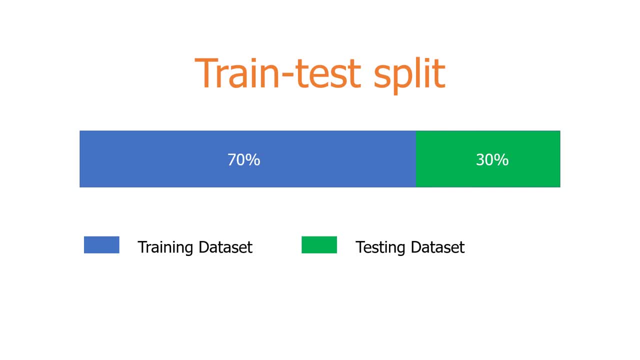 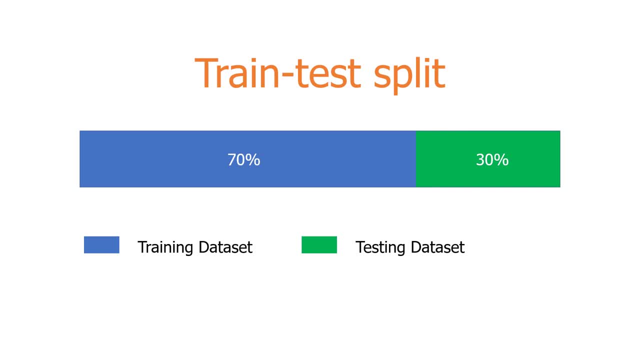 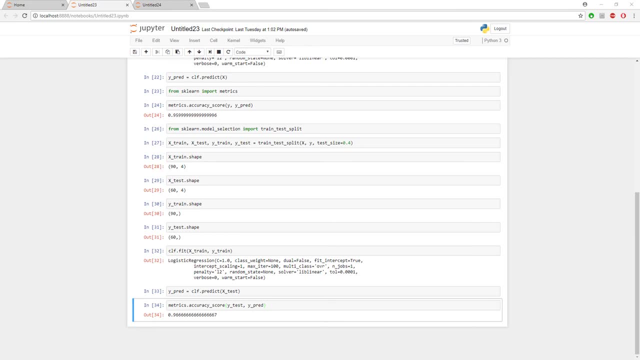 very high variance estimate of out of sample accuracy. so let me go to my jupiter notebook and explain you what do i mean by that. so note that now the accuracy is 97 percentage and this train test split method randomly allocates the observations into a training set or a testing set. 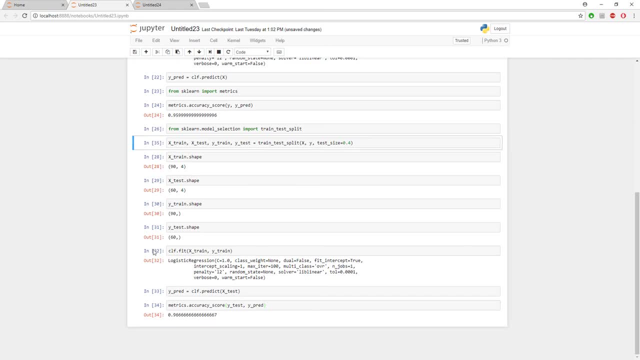 so if i execute the method again and try to fit the data and get the predictions and calculate the accuracy score, you see that the accuracy has fallen down to 93 percentage. so that's what i mean by saying that train test split produces what is known as a high variance. 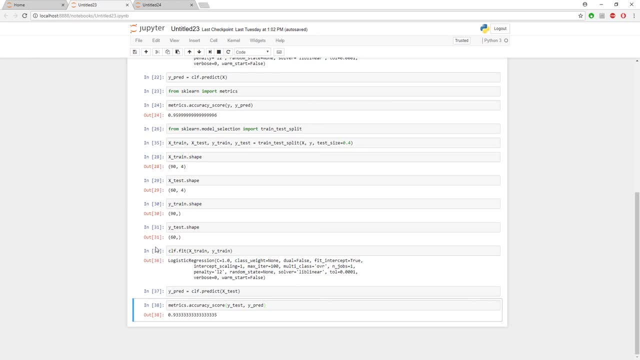 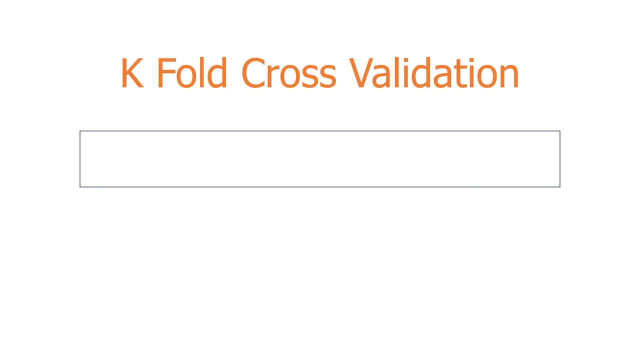 estimate. the real estimate basically depends on which set of observations are there in the training set. so you cannot meaningfully rely on a train test split method to produce accurate results. so blihe might wonder what if we created a bunch of train test splits, calculated the testing accuracy? 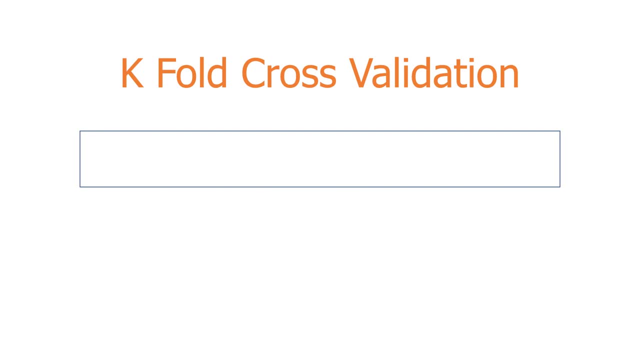 of each and average the results together. and that is the essence of the third method of evaluation, which is called the k-fold cross validation. so in k-fold cross validation we split the data set into k equal partitions or folds. the k value can be anything. here i have taken the k value to be as 10. 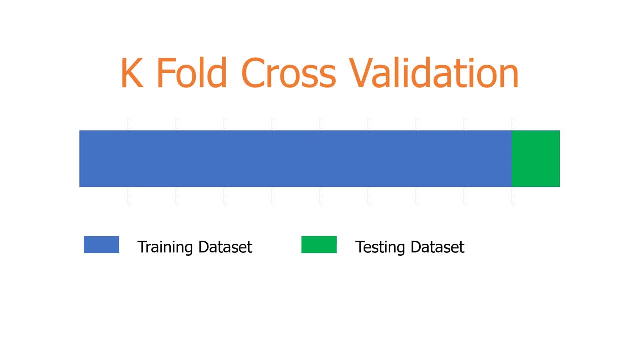 Then we use the fold one as the testing set and the union of the other folds as the training set, and then we calculate the testing accuracy. We repeat this step for 10 times, or k times each time, calculating the accuracy score and averaging the accuracy score of all the 10 different instances. 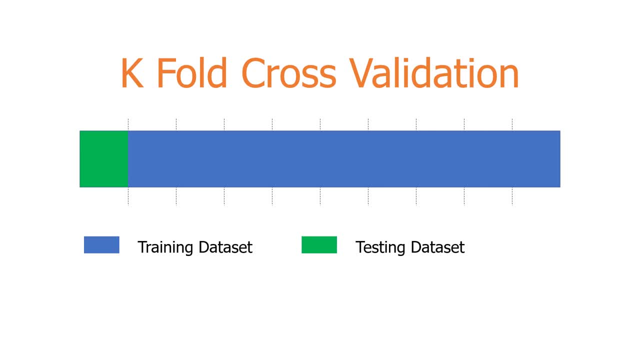 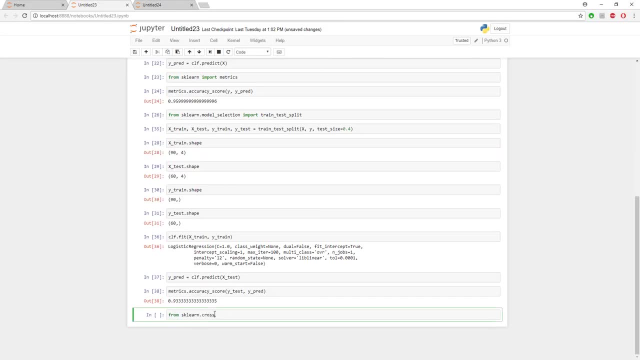 And the average testing accuracy is used as the estimate of out of sample accuracy. So first let me import the crossval score module from sklearncrossvalidation And I will go and execute the function crossval score and store the output of that function in a variable called scores. 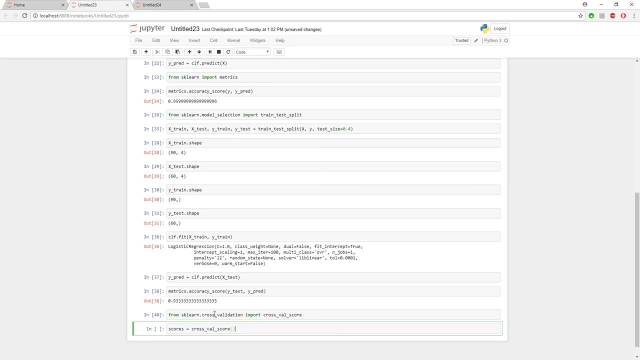 This variable scores is an array and it holds the result of each of the 10 different iterations of a validation that we are going to do. So within the crossval score, I need to pass in an estimate, Which can be anything. it can be instantiated to either random classifier or logistic regression. 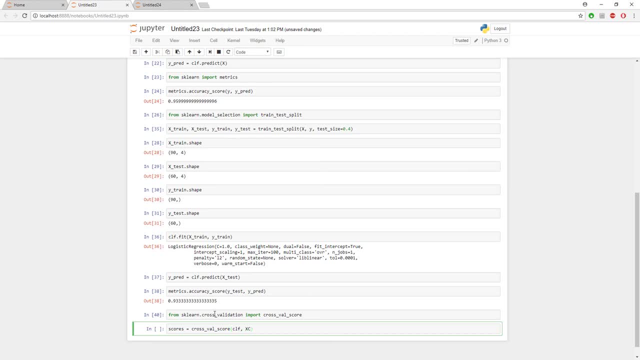 or knn, And then I need to pass in my x and y values and I need to say what are the different number of folds that my data set has to be divided into. So basically I was using 10 folds in the slides, So I will give cv as 10 and then I need to score this for accuracy.